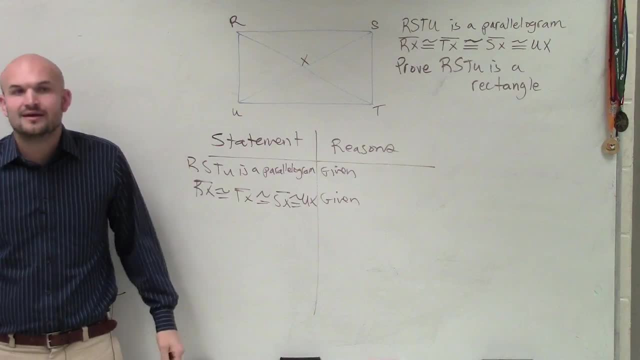 Yes, Yes, But we've got to be able to show it has four right angles. And last class some students said: well, why don't you just put a nine degree symbol in there, Right? Well, that's like me telling you. 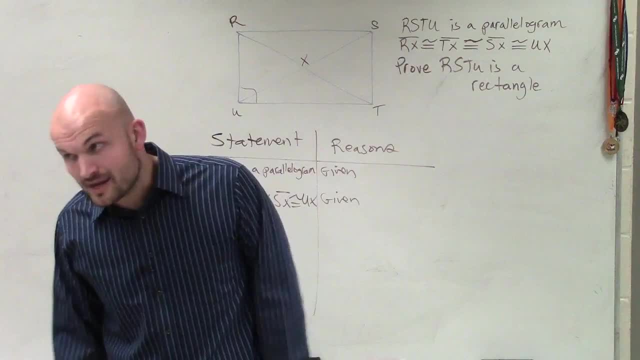 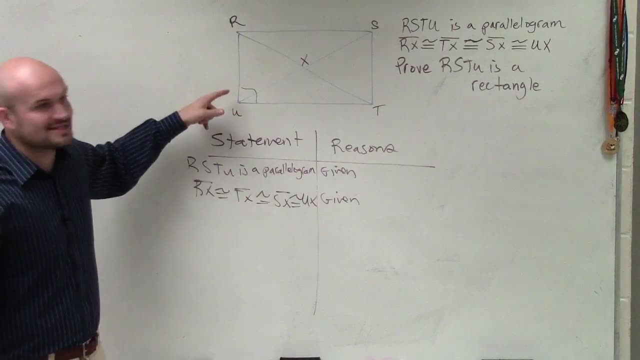 Hey, I only weigh a hundred pounds. I don't weigh a hundred pounds, Right? But if I tell you I weigh a hundred pounds, that's what I'm telling you, Right? You don't know, this is 90 degrees. So you just can't say, oh, it's 90 degrees. That's like me just saying, oh, I weigh a hundred pounds, Right. 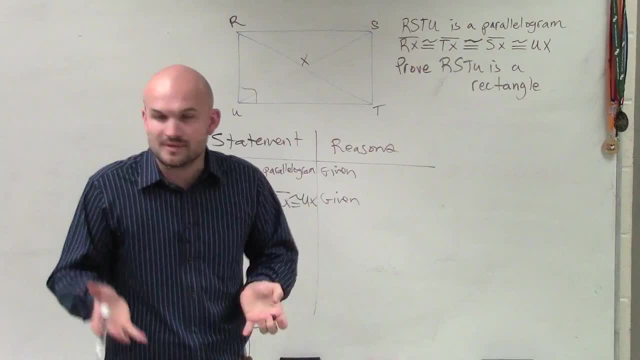 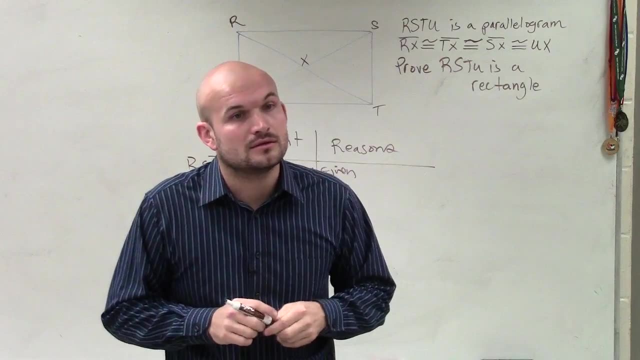 You've got to be able to measure it or use some type of theorems or something that you can use, Right Tyler, To be able to show that it's worth 90 degrees. Yes, Is it a definition of a rectangle? 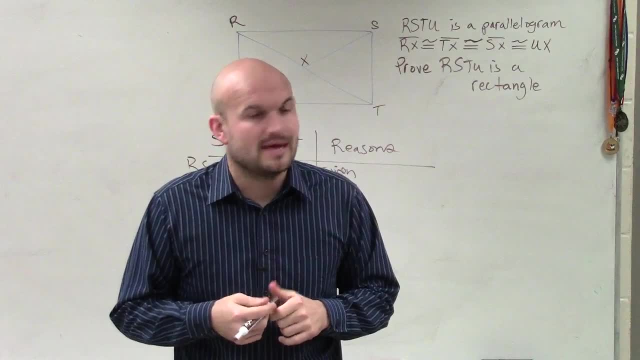 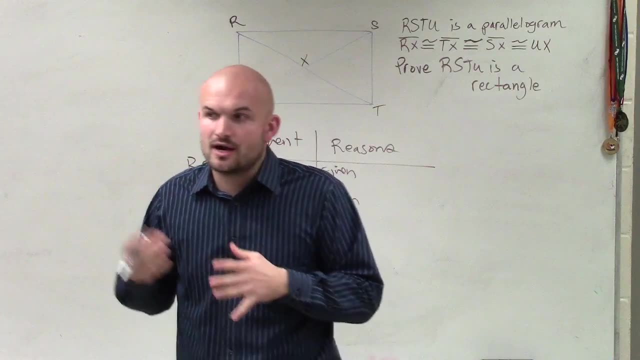 Yeah, but we don't know. it's a rectangle, though. yet We're trying to prove it's a rectangle. That's our problem, That's our issue right now. So we need to think all right. so maybe right angles might be a little difficult for us to be able to show with what we know. 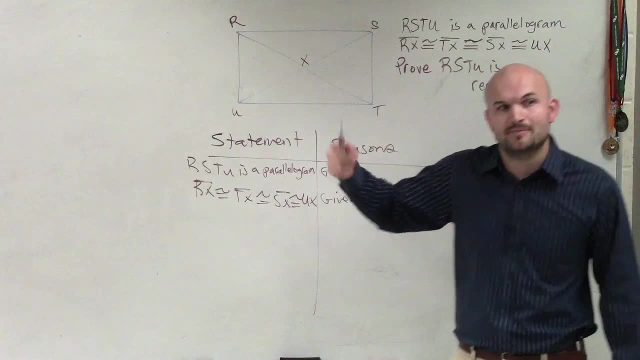 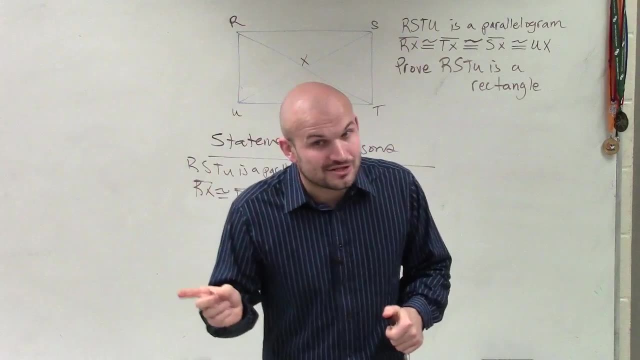 Because the only thing we're given is that sides are equal to each other. Does anybody else know what else is unique about a rectangle? Yeah, Colin, again, Diagonals bisect each other. Diagonals bisect each other, but parallel guns bisect each other. Something else: 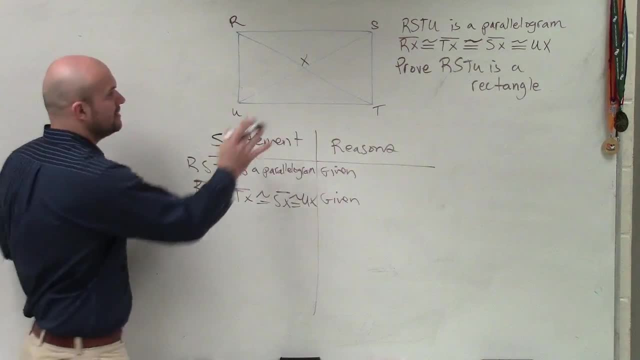 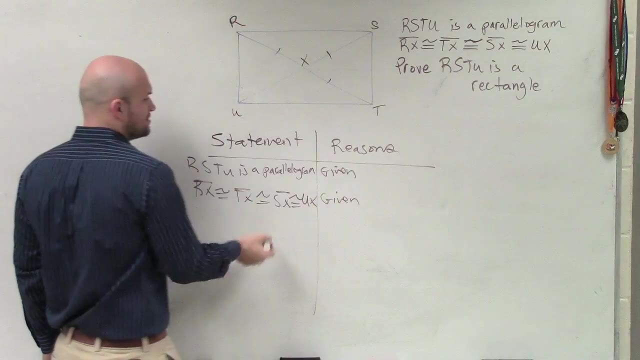 Yes, Diagonals are equal in measurement. All right, Now let's go and look at what we have here. We already they say that RX is congruent to TX, which is congruent to SX, which is congruent to UX. Right, 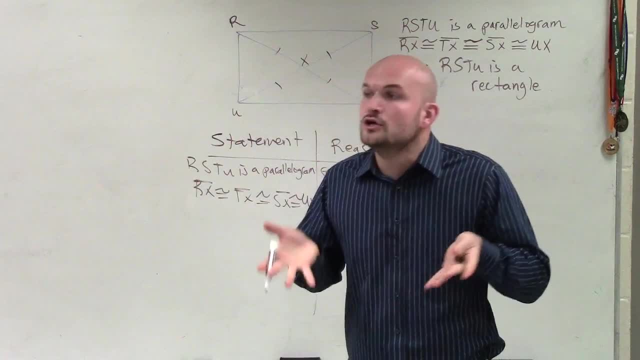 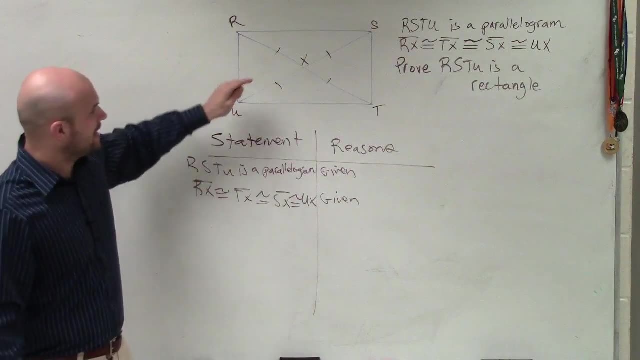 But remember to show that- excuse me, to show that the diagonals are equal in measurement. we've got to be able to show that they are. to be able to show that it's a rectangle, we've got to show that the diagonals are equal in measurement. 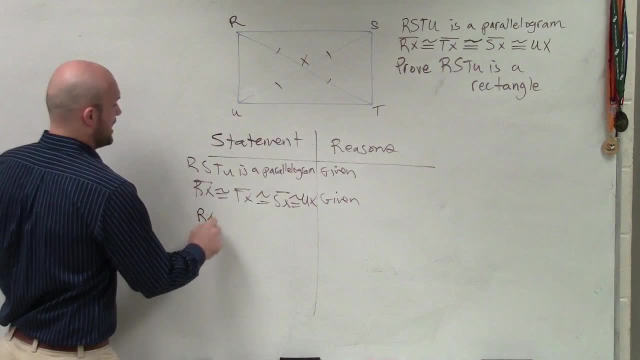 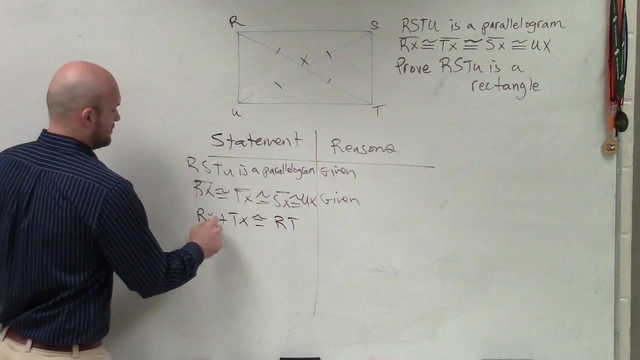 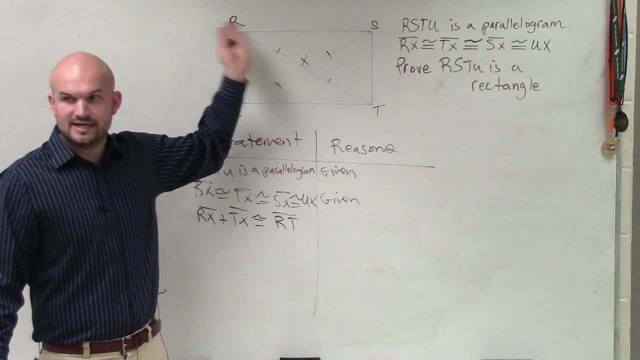 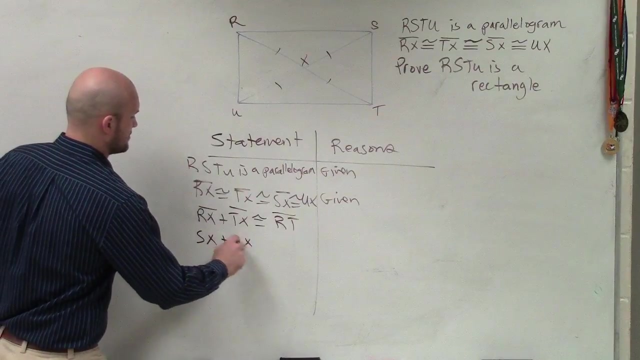 So the next thing I would say is: RX plus TX is congruent to RT. Would you guys agree with that? The sum of these two lines equals the whole line. Yeah, And then I would also say that SX plus UX is congruent to. 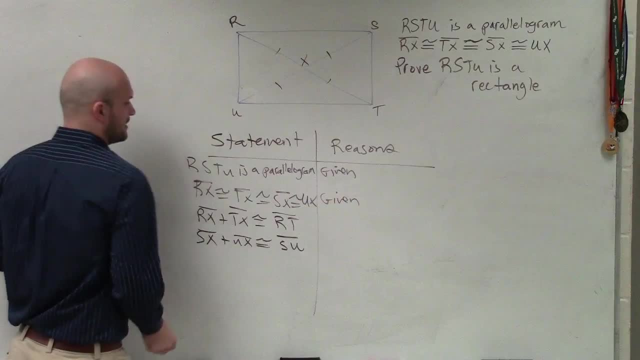 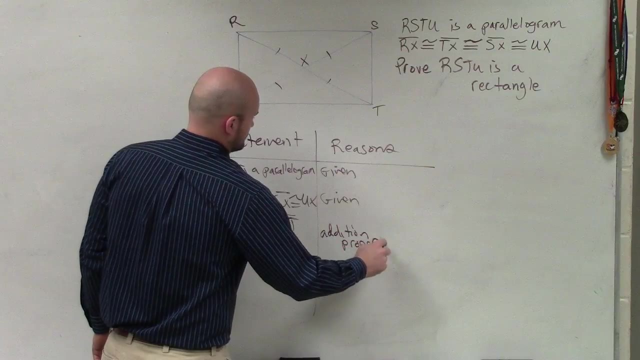 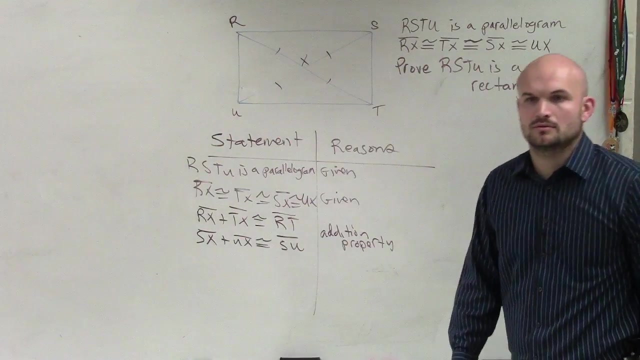 SU, SU. And why do we know that? Well, that's just because of the addition property. Just add them up. Now, Josh, I'm going to ask you very politely to put that down, so you can write down this. So now, what do we know? 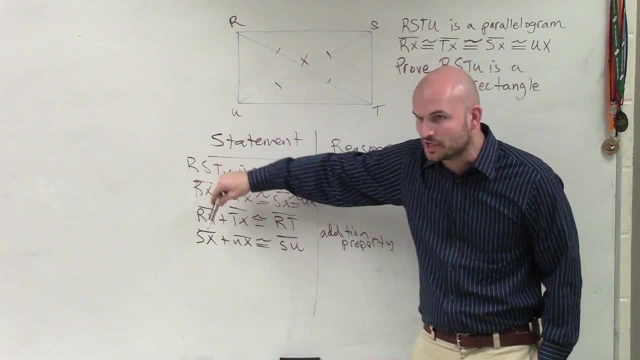 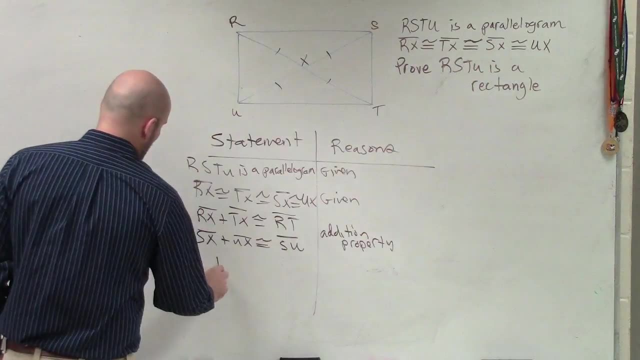 If these two add to this and these two add to this, and these are all equal to each other. does it make sense then that these two are equal in measurement? Yeah, So now we can say that RT is congruent to SU. 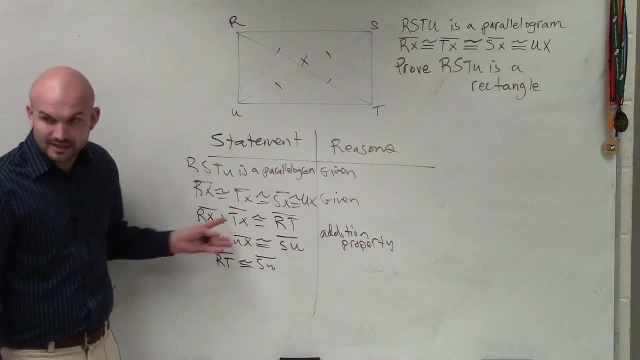 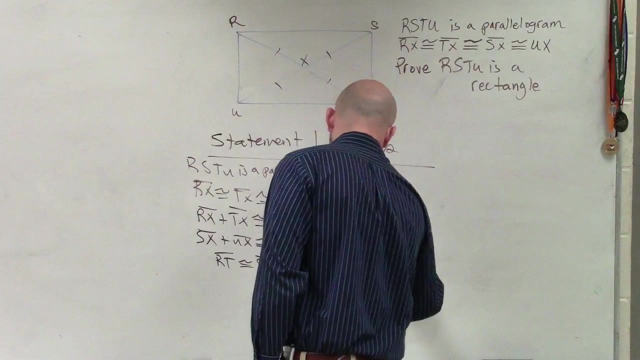 All right, Because all we're doing is we're substituting in these values. So I'll just go ahead and say that, a substitution, that because, since these sides are equal, all equal, and they add up to different sides, but those sides are not equal. 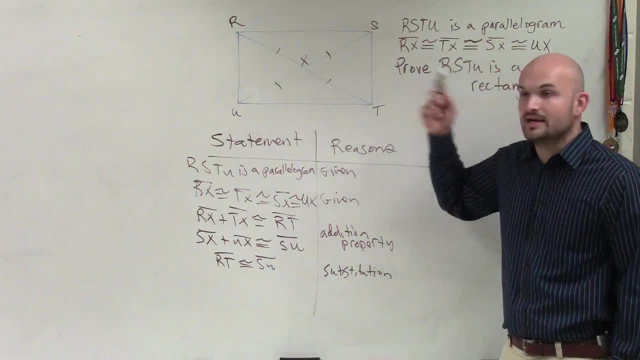 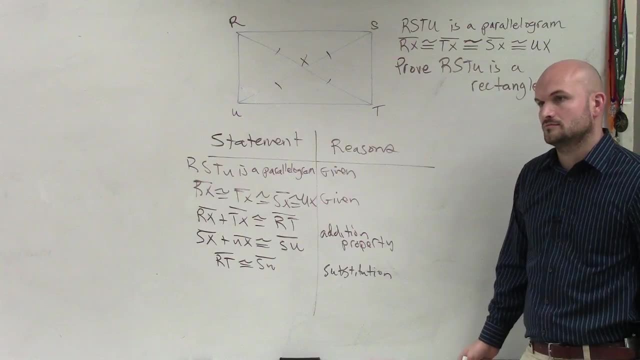 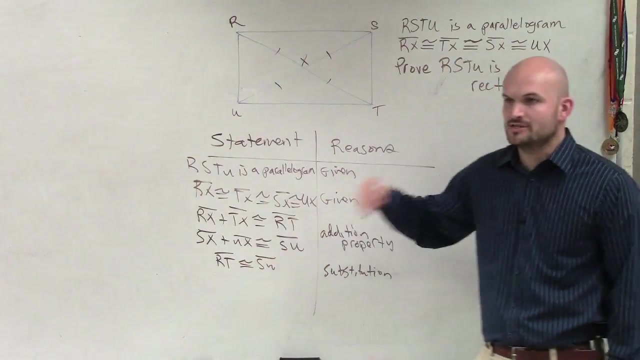 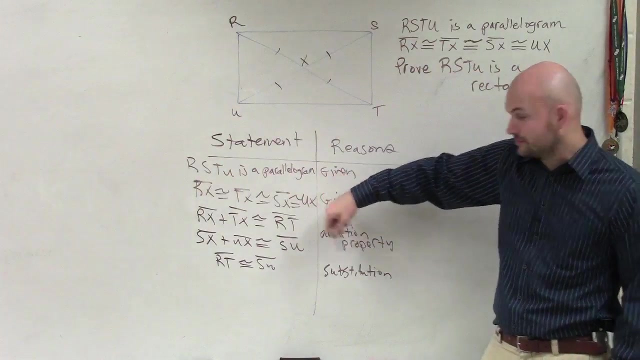 they're now going to be equal. And then now, Yes, Yeah, that's right, But you're not adding these two. You're not adding these two sides. You're saying these two sides are equal in measurement, But the reason you get this is for your addition property. 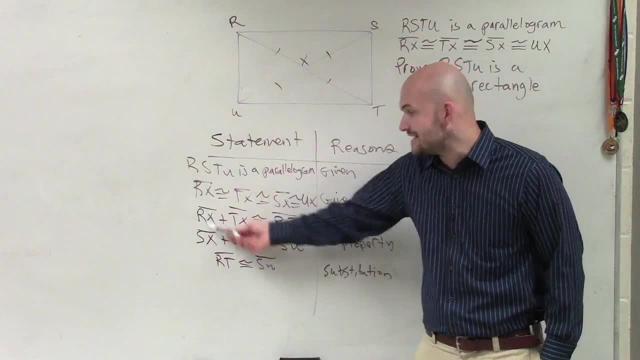 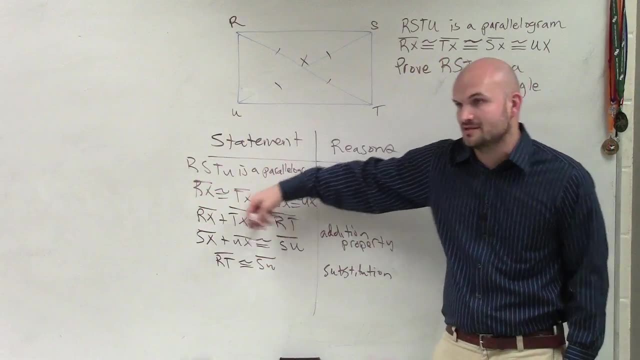 The reason that these are equal to each other is because, yeah, all these sides are equal and all these sides. So you're substituting the sum equal, these two sides, So you're like substituting the sum of these two in for these two lengths. 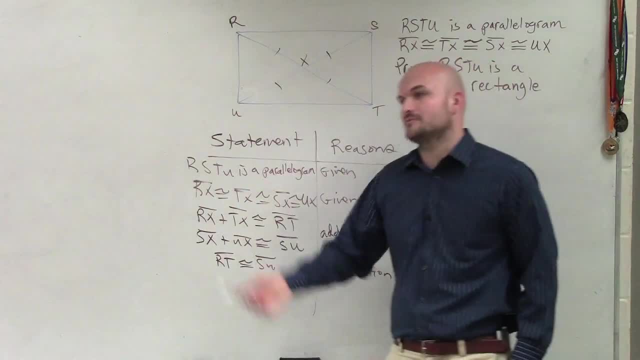 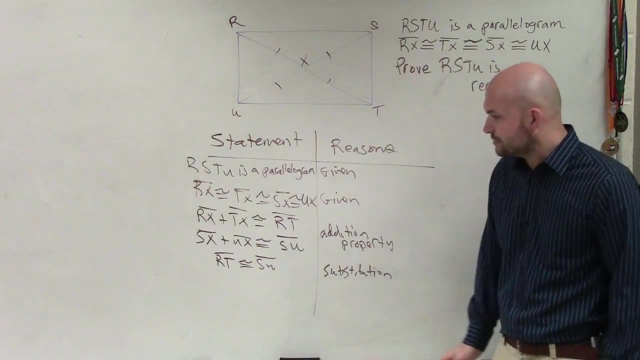 and that's why it equals that side. All right, And again, remember on, like you know, especially like on a multiple choice, you'll have options. you know of different properties you look at that you can be able to use. 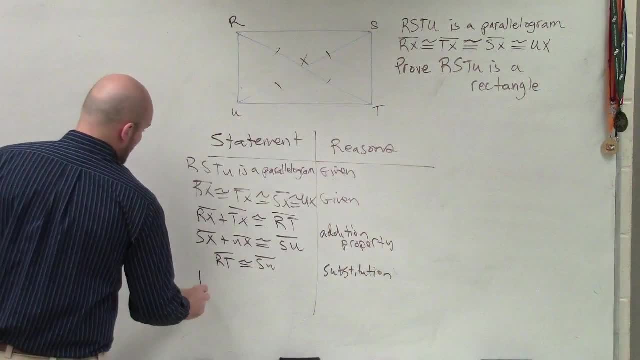 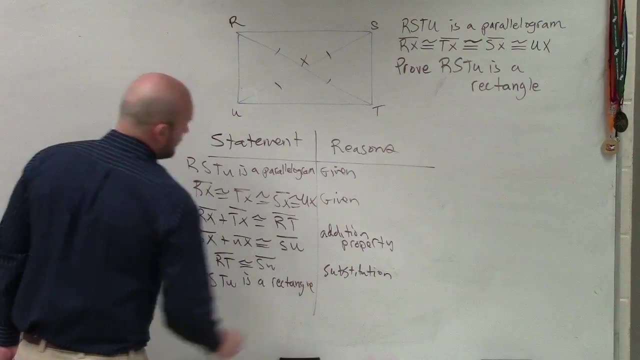 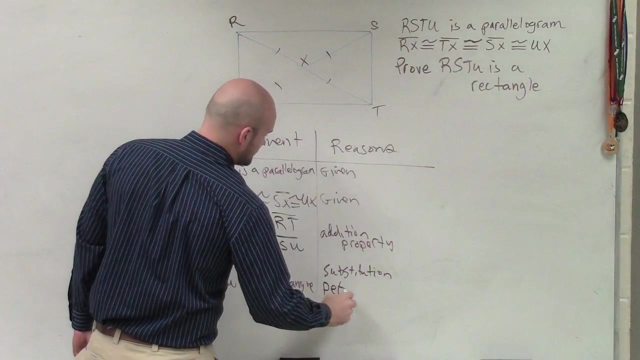 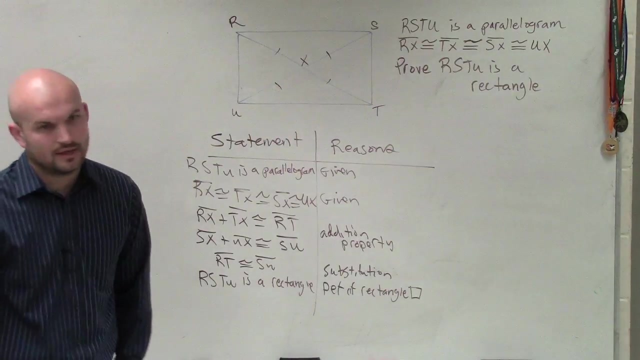 And then on. the last thing is now I can say that RSTU is a rectangle. Well, why is it a rectangle? Well, because your diagonals are equal to each other, which is part of the definition of a rectangle. And there you go. 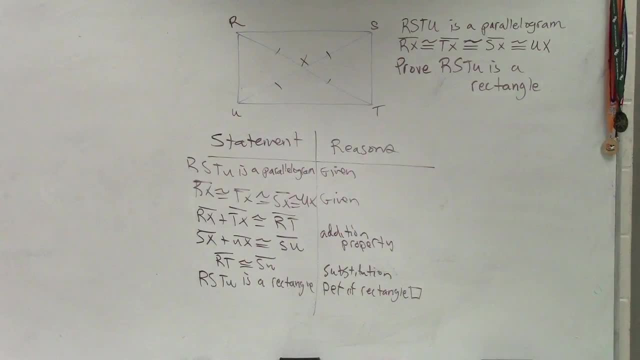 There you go Now. I just did your proof for you. That's so nice, doesn't it? Done like every.